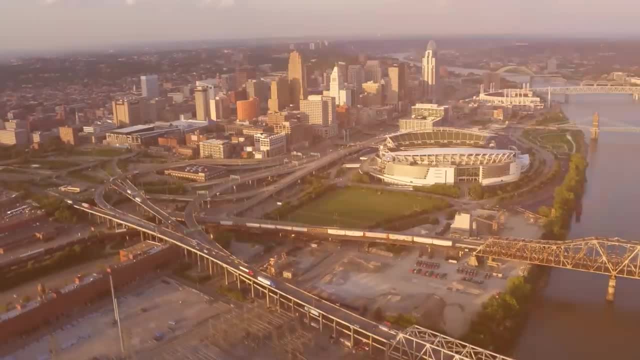 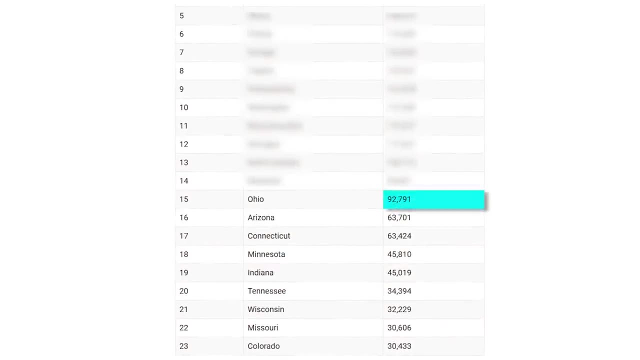 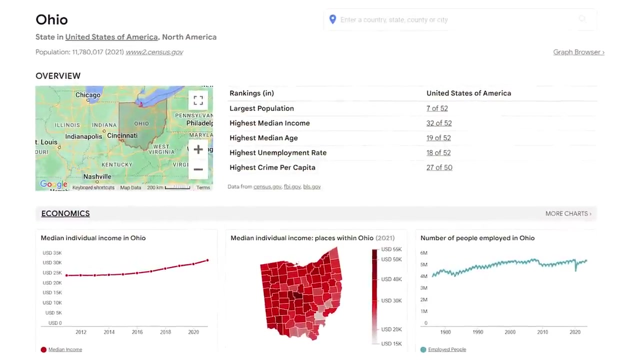 in Number 15, Ohio. The state with the 15th highest Asian Indian population is Ohio, which has a population of just under 100,000 Indian people, or 92,791.. This is compared to the state's population of about 11.7%. 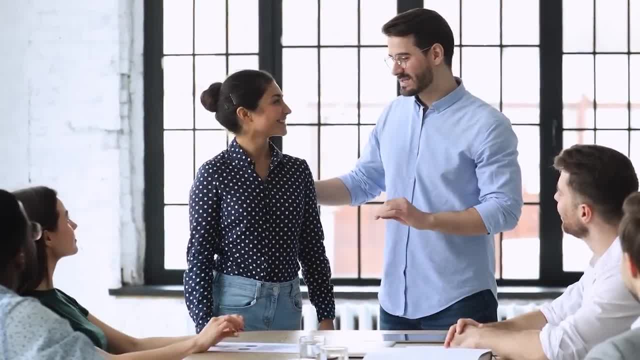 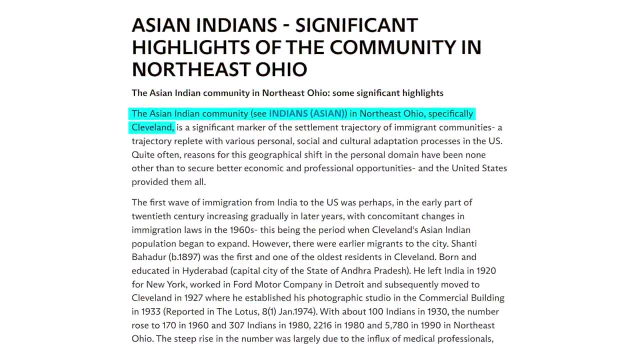 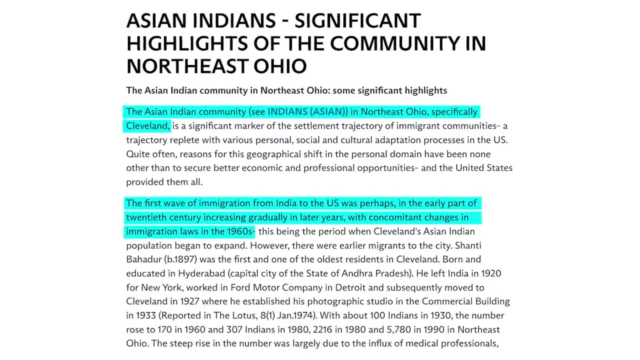 78 million, meaning that its Indian population makes up about 0.79% of the state's total residents. Many of these people live in Northeast Ohio, and specifically in the Cleveland area, where the Indian population first began to see an increase in the 1960s after the Immigration. 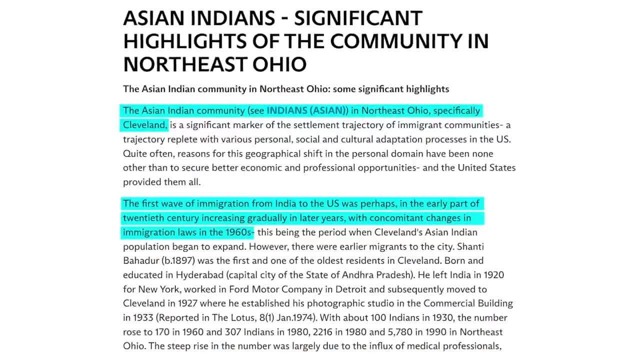 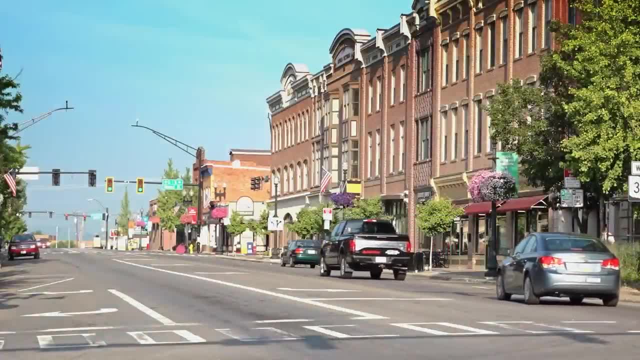 and Nationality Act of 1965 first started allowing graduate students and professionals to come to the US from other nations. Since then, Indian people have continued to reside in this area and they've been living in the US for a long time. They've been living in the US. 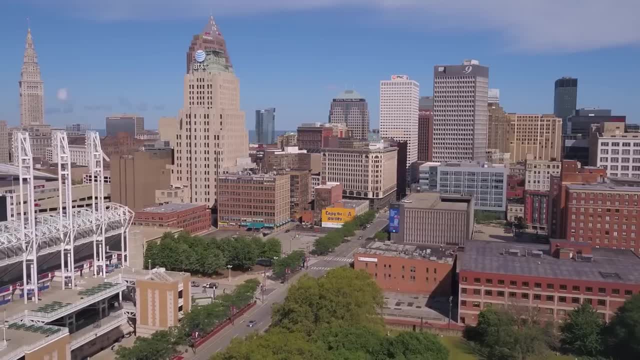 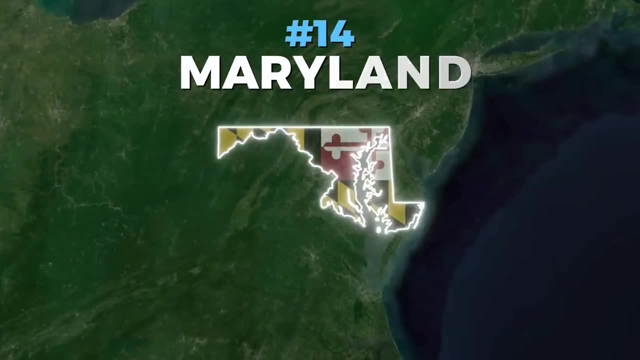 area, either to continue their education or training or to find work in one of Cleveland's numerous medical institutions, universities or business firms. Number 14,, Maryland. Number 14 is Maryland which, as of the latest census count, had about 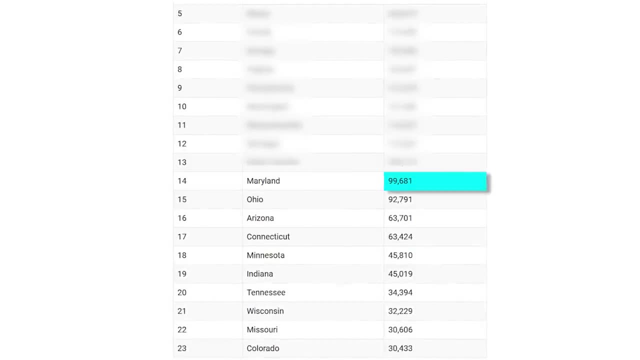 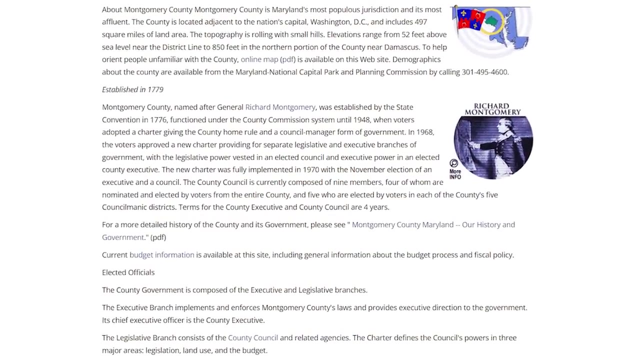 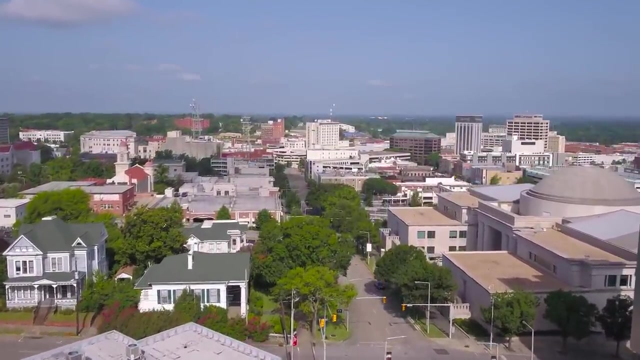 100,000, or 99,681 Asian Indian residents. Many of these people live in Montgomery County, which is a suburb of Washington DC. As you can imagine, the reason for living in Montgomery County is that it's within close commuting distance to the numerous jobs. 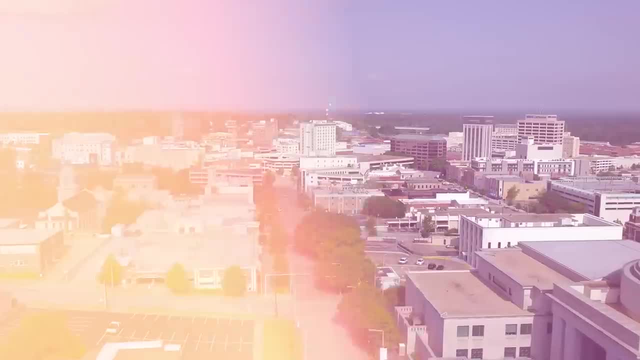 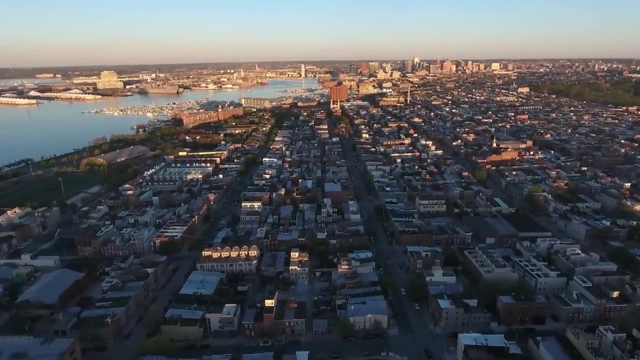 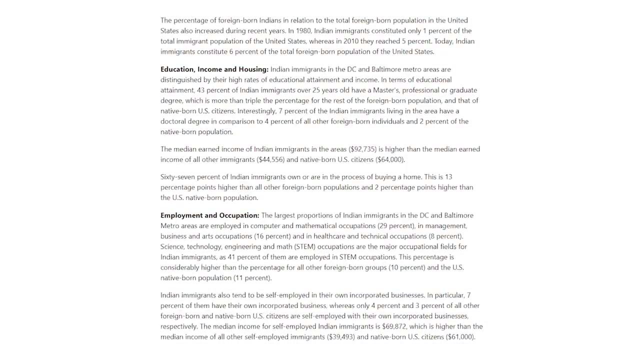 available in the Washington DC metropolitan area. In addition to Washington DC, another popular area is the Baltimore area, although fewer Indians live here than in the DC suburbs. According to data from George Mason University, many of the Asian Indians who live in Maryland 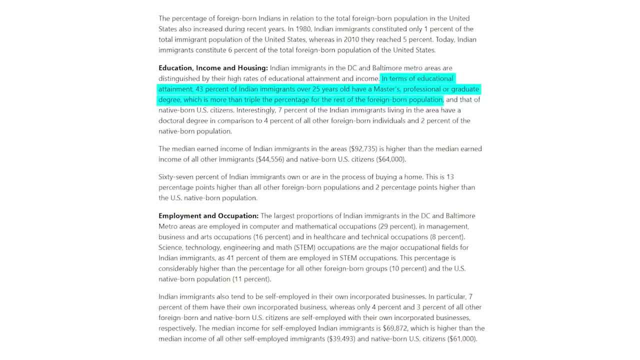 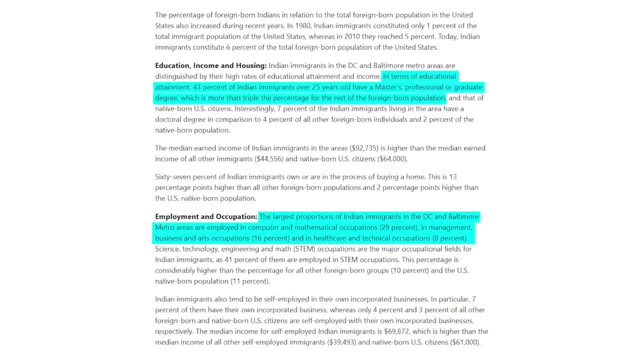 are highly educated, with 43% having a master's, professional or graduate degree, which is about triple the overall rate. Additionally, those who settle down here tend to work in the computer and math fields, with 29% working in this industry. Management. business and arts is a close second, with 16% working in these occupations, followed by healthcare and technical jobs at 8%. Number 13, North Carolina. Approximately 105,712 Asian Indians live in North Carolina, putting it at number one. Number 12, North Carolina. Number 13, North Carolina Number. 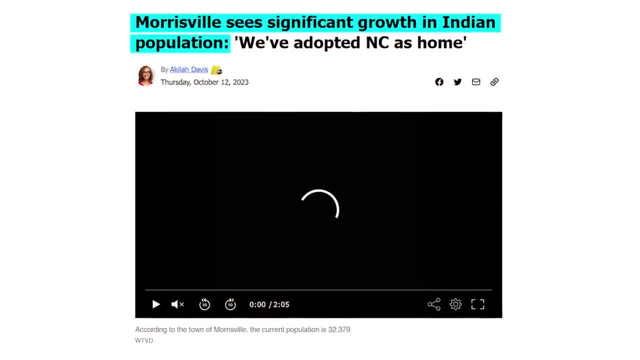 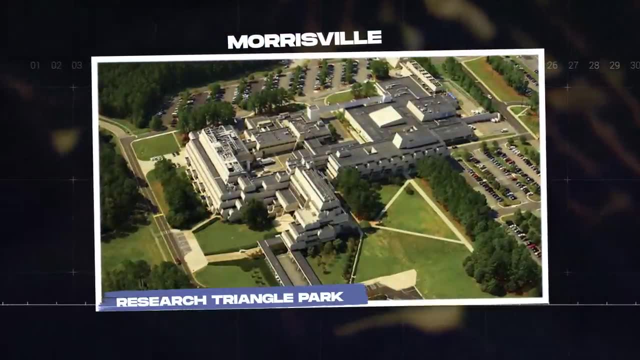 13 on our list. Morrisville in particular has seen a significant increase in its Indian population. If you're not familiar with Morrisville, it's part of the so-called Research Triangle or Research Triangle Park, which is named for the area connected by Duke. University, North Carolina State University and the University of North Carolina, Chapel Hill. While the total population of Morrisville is only about 31,000, those from India and other Southeast Asian countries are the largest representative of the Indian population. As you can imagine, many of those people are drawn here due to the educational and work. 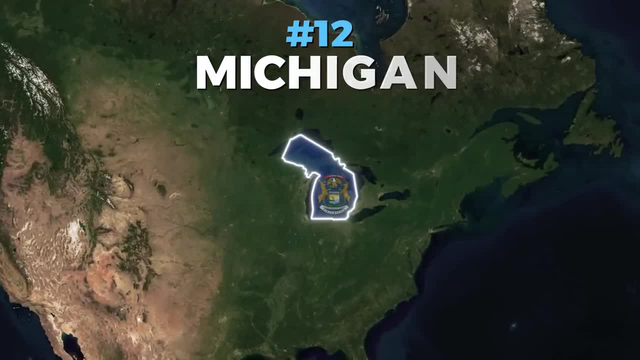 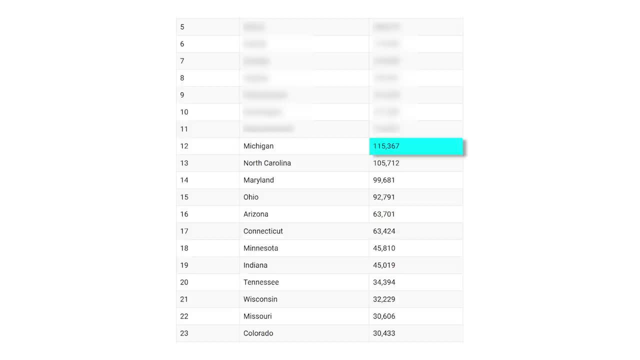 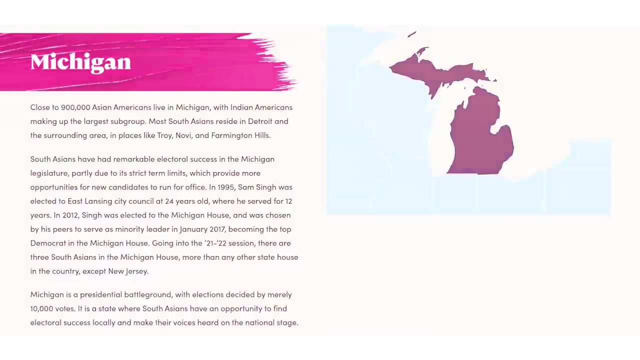 opportunities in the Research Triangle, Number 12,, Michigan. As of the latest census count, Michigan has about 115,367 Asian Indians living there. That's compared to its total population of about 10 million people According to Indian American Impact or. 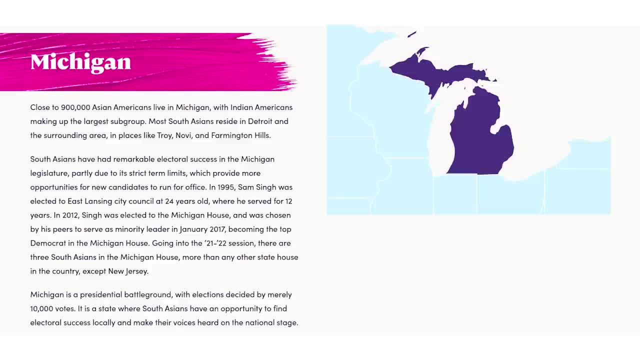 IAEA. Michigan has about 115,367 Asian Indians living there. That's compared to its total population of about 10 million people. Number 11,, IA Impact, A non-profit that seeks to empower South Asian and Indian American populations. Indian Americans actually make up the largest subgroup of Asian Americans living 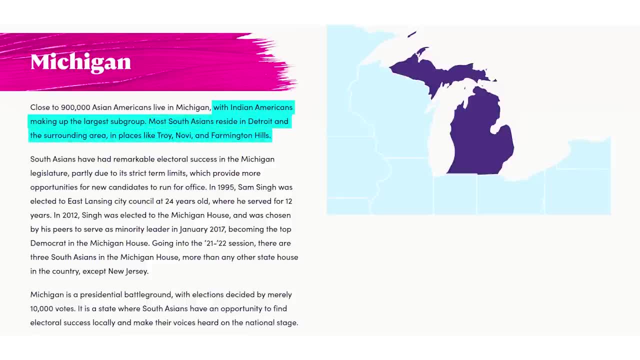 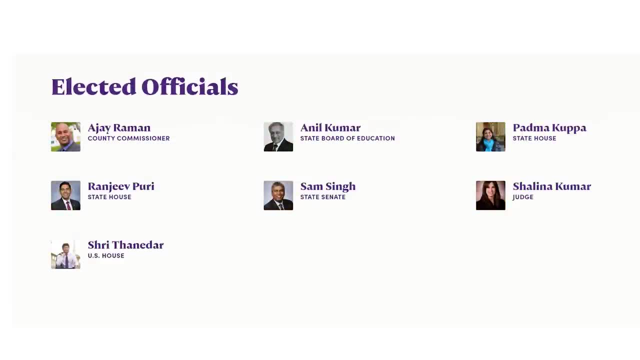 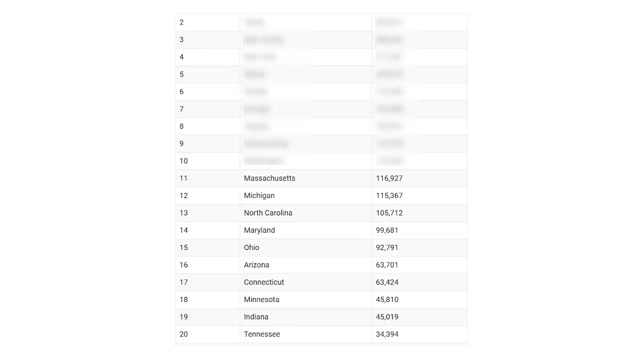 in Michigan. Most of these people live in Detroit and its suburbs, likely due to work opportunities there. IA Impact also notes that Indian Americans have made a name for themselves in Michigan politics, with representatives like Sam Singh finding a place in the Senate. Number 11, Massachusetts. Number 11 is Massachusetts, which has an Indian population. 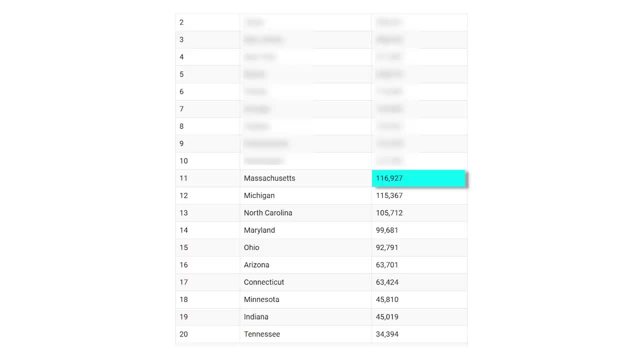 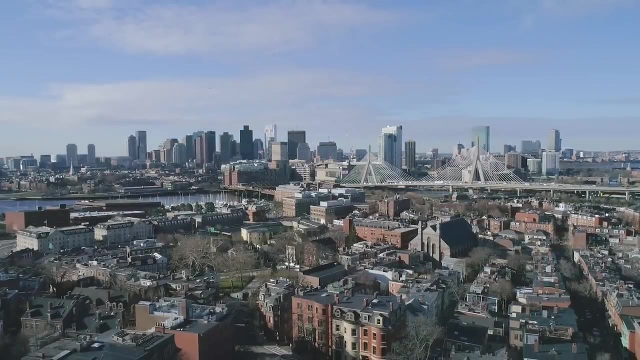 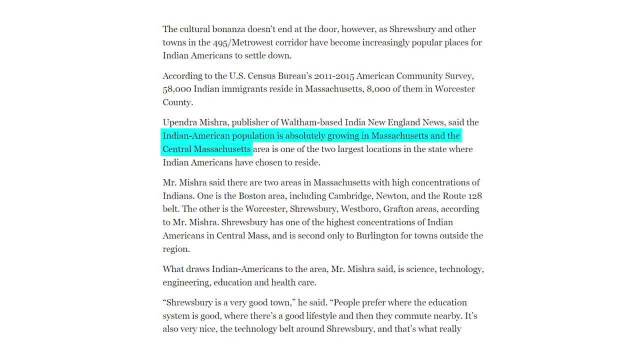 of approximately 116,927,, which is about 1.7% of its total population of about 6.9 million. Apparently, the state's Indian population has been growing for quite some time now, with these centers of growth concentrated in the Boston and the central Massachusetts areas. 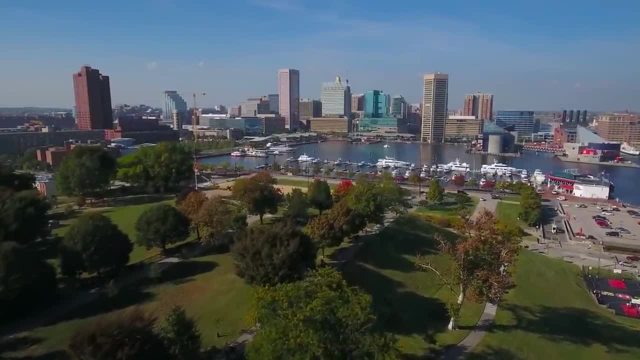 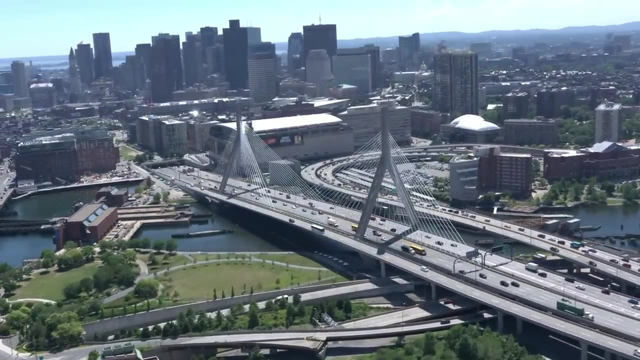 Like we saw with those in Maryland, Asian Indians living here also tend to be highly educated, with a 2017 article noting that about 50% of those located in the Boston region between 1990 and 2000 had graduate or professional degrees. Number 10, Washington. Washington state has about 127,282 Asian Indian residents. As we've seen so far, most of these people tend to be clustered in the state's urban regions like Seattle, Likely for work and educational opportunities. Interestingly, the Indian population is growing. 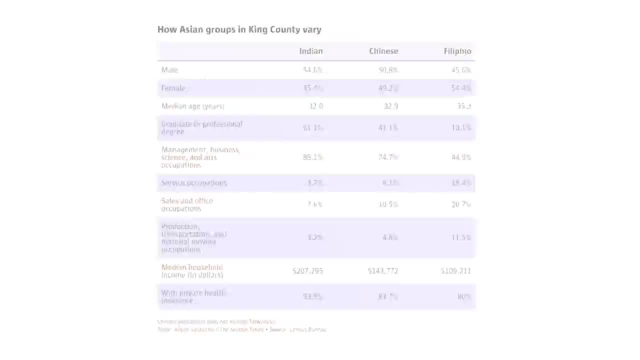 quickly here doubling in the past decade alone. About 61% of those Indians who live in the Seattle area hold a graduate or professional degree and an overwhelming majority- about 85%- work in management, business, science and arts occupations. Additionally, the median household income is significantly higher than that of the Seattle area as a whole, at a median income of $207,295, compared to the overall median of $116,340.. Number 9, Pennsylvania. Next up is Pennsylvania, which had an Indian population of approximately. 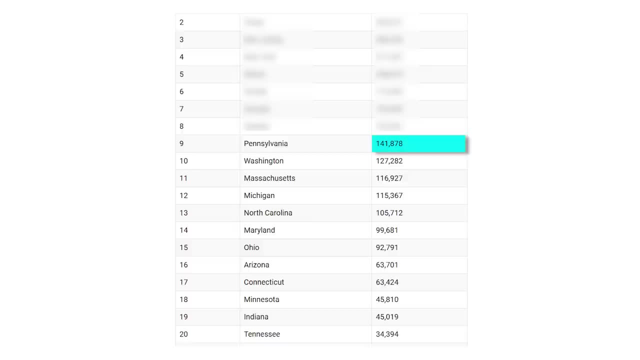 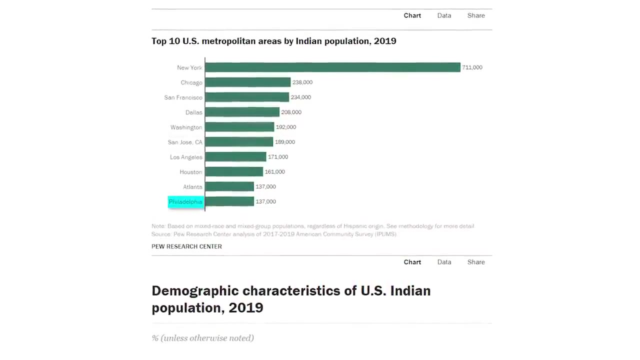 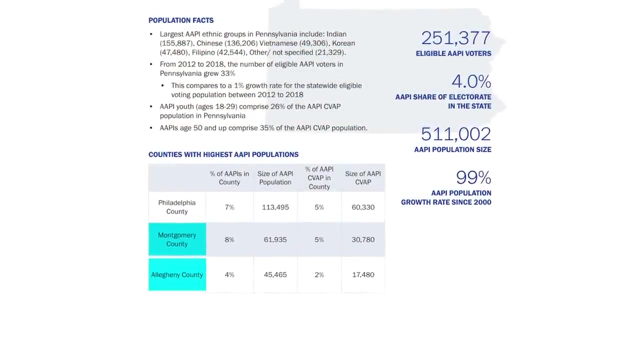 141,878, as of the latest Census count. Notably, Philadelphia is among the top 10 US metropolitan areas with the highest Indian populations. In addition, Montgomery County, adjacent to where Philadelphia sits, and Allegheny County, which is the home of 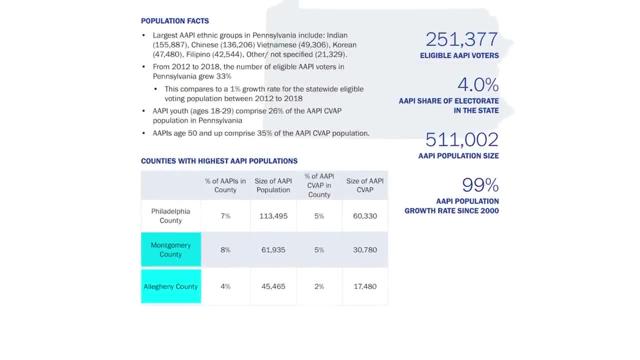 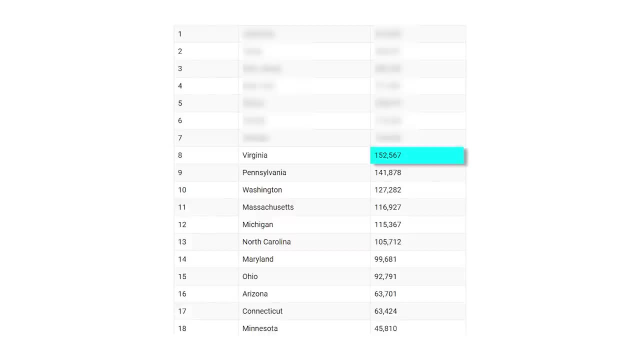 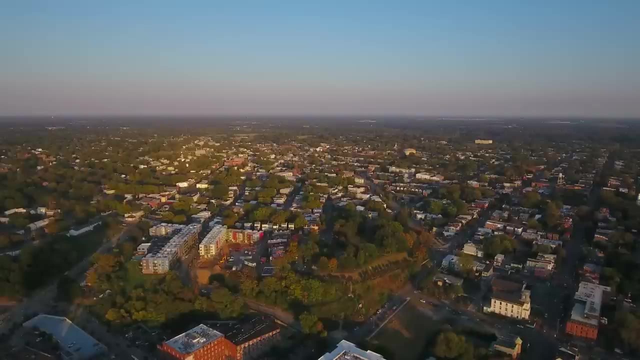 Pittsburgh also have significant Indian populations. Number 8. Virginia: Virginia has an Asian Indian population of approximately 152,567, compared to its total population of about 8.6 million. That means that Indians represent about 1.8% of the state's total. 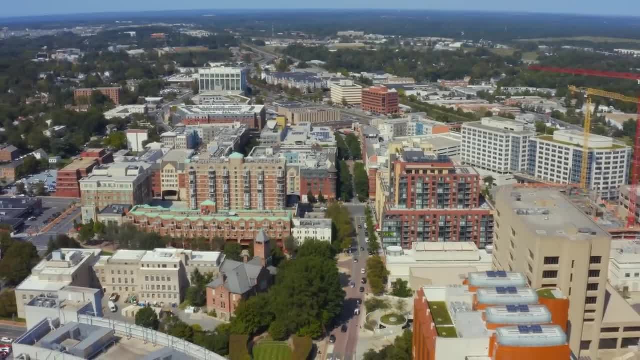 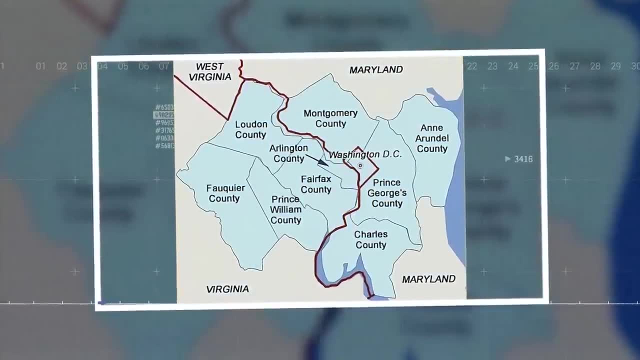 population. Interestingly, we see a lot of parallels here with another state we looked at Maryland. That's because several areas in Virginia are also suburbs of Washington DC, meaning that people tend to move there due to the jobs and educational opportunities provided by DC. 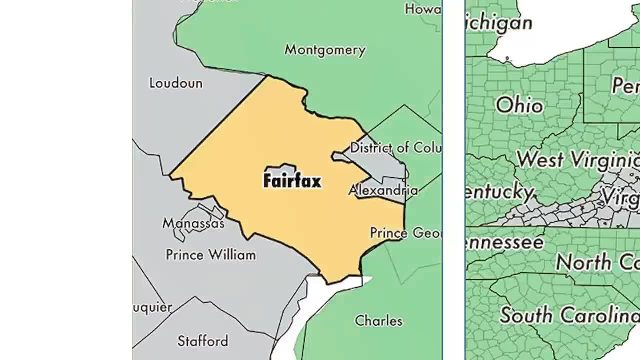 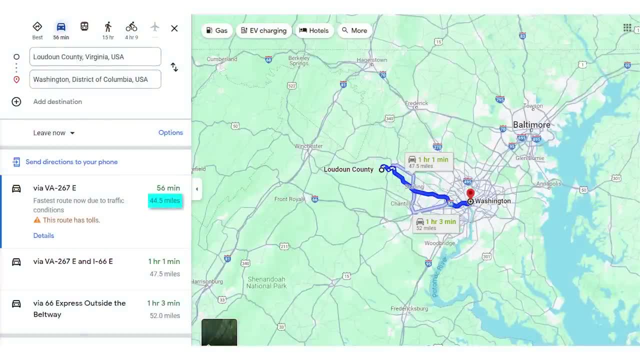 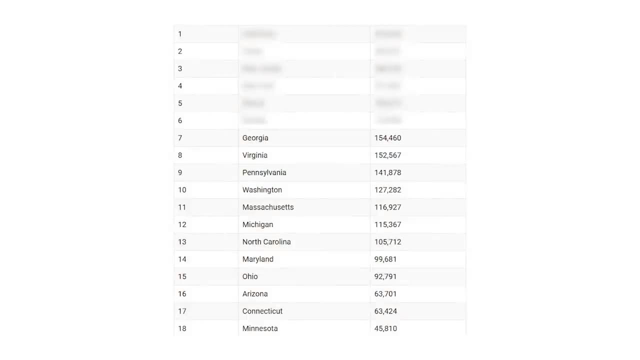 For instance, a significant number of Indians live in Fairfax County in Virginia and in Loudoun County, which, for reference, are about 21 miles and 45 miles outside of Washington DC respectively. Number 7. Georgia- Georgia comes in at number 7 on our list with 154,460 Indian. 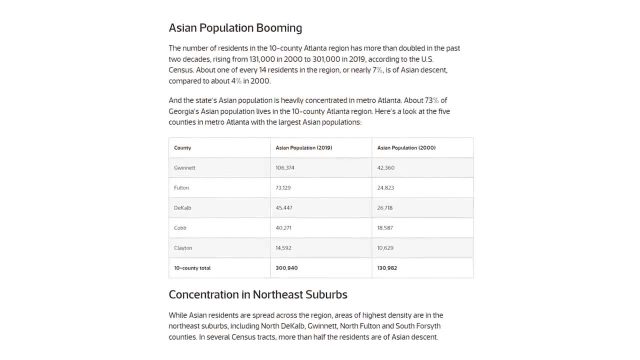 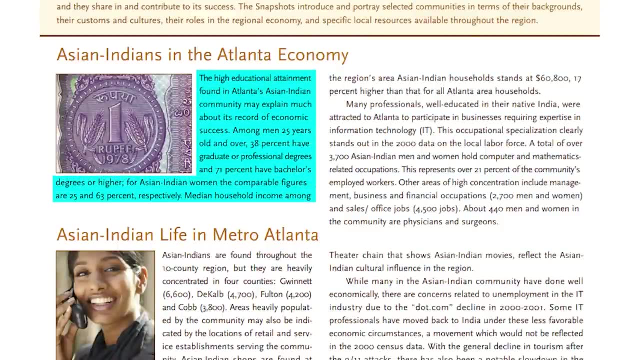 residents there. This population is growing quickly, with a lot of people settling down in the Atlanta region in particular. Like we've seen elsewhere, this population tends to be highly educated and hold solid jobs. For instance, 38% of Asian Indian men and 25% of Asian Indian women. 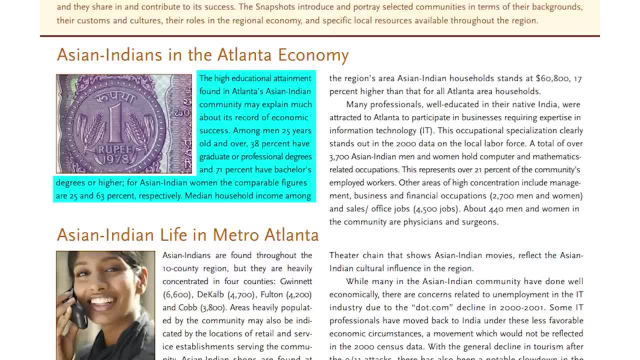 have graduate or professional degrees, while 71% and 63% have bachelor's degrees respectively. The median household income for Indians in the Atlanta region also tends to be high, at a number that's 17% higher than the overall median. Those working in the region tend to work. 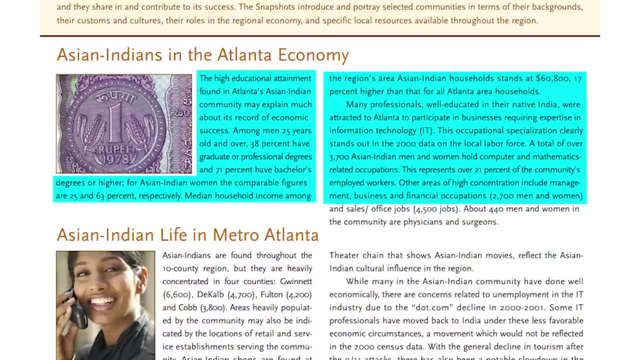 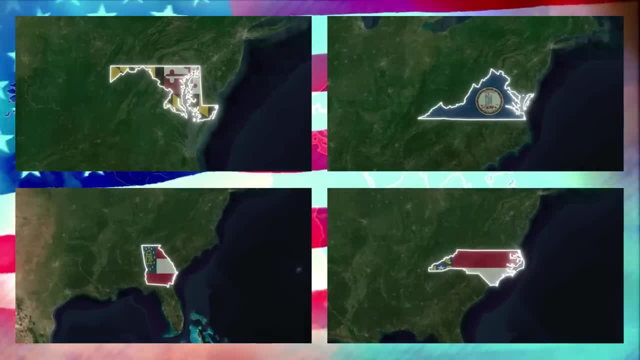 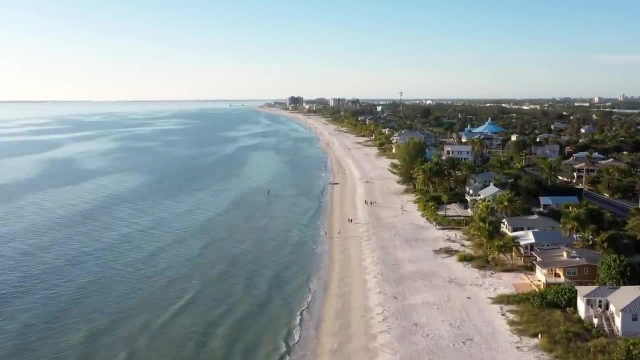 in tech and science-related jobs, along with management, business and finance. Number 6. Florida. In addition to Maryland, Virginia, Georgia and North Carolina, Florida is yet another South Atlantic state that has attracted a relatively large Asian Indian population. In fact, there are 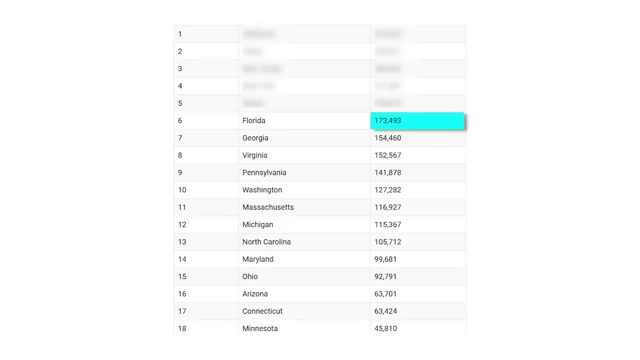 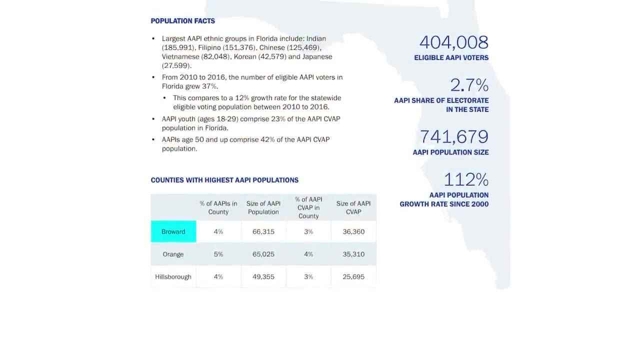 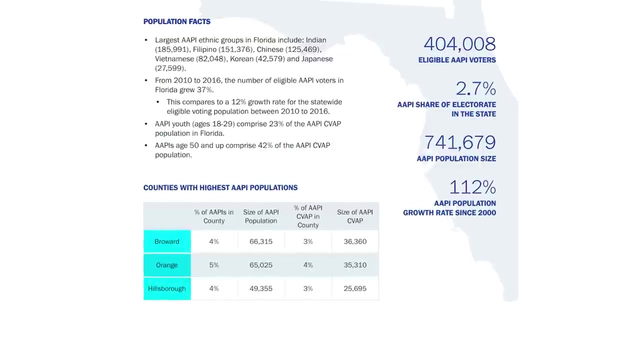 173,493 Indians here, according to the latest census numbers. Most Indians who live in Florida are clustered in Broward County, which is where the city of Fort Lauderdale is located, along with Orange County, where Orlando Orlando is, and Hillsboro, home to Tampa, among other small cities. 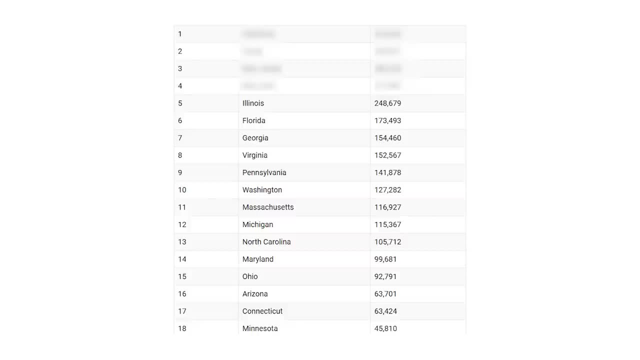 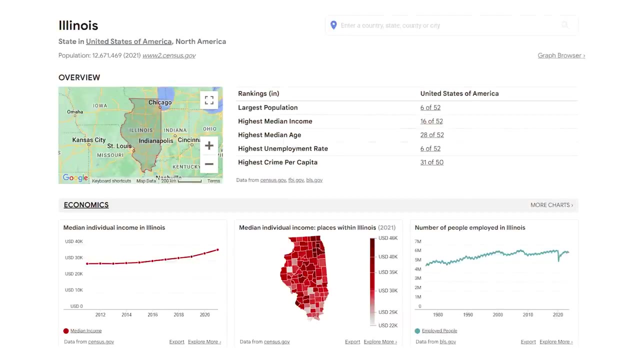 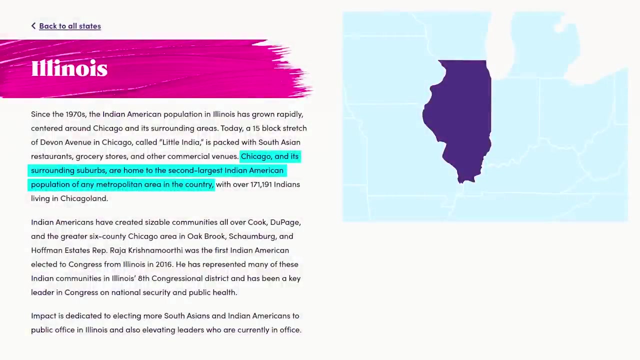 Number 5. Illinois. Illinois has about 248,679 Asian Indians living there, compared to its total population of about 12.67 million. Most of these people live in the Chicago area, which has the second largest Indian American population out of any other metropolitan area in the entire country. Chicago even has a 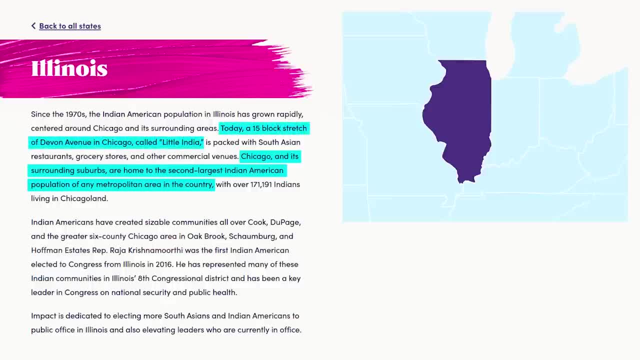 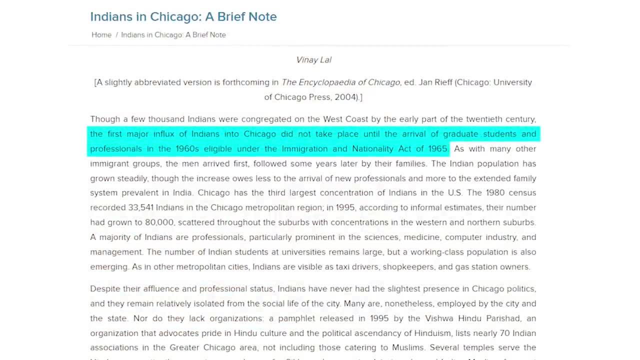 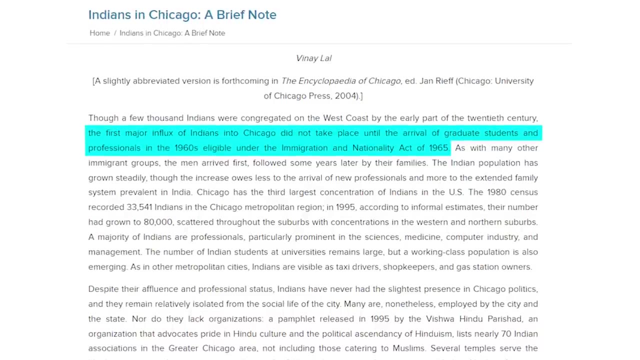 15-block stretch of restaurants and shops, fondly known as Little India. Similar to what we saw in Ohio, Asian Indians started coming to this region when the Immigration and Nationality Act of 1965 began allowing graduate students and professionals to come to the US. Today, in addition to a large 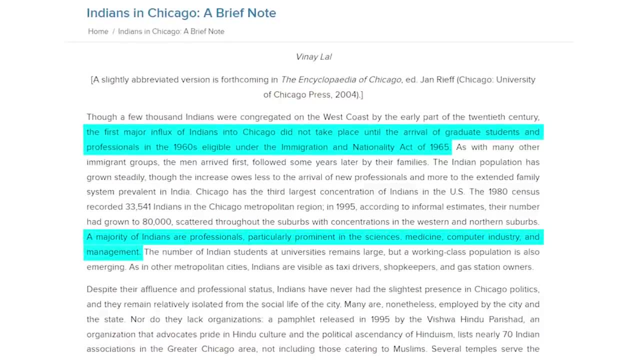 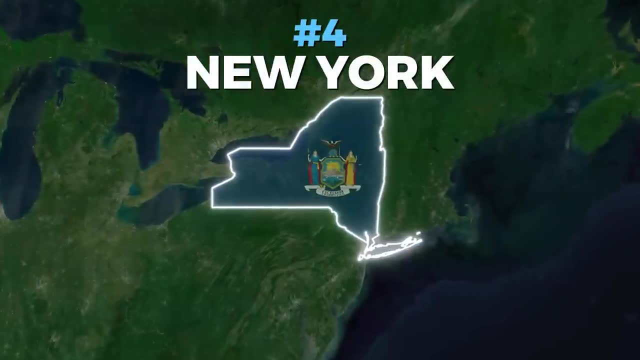 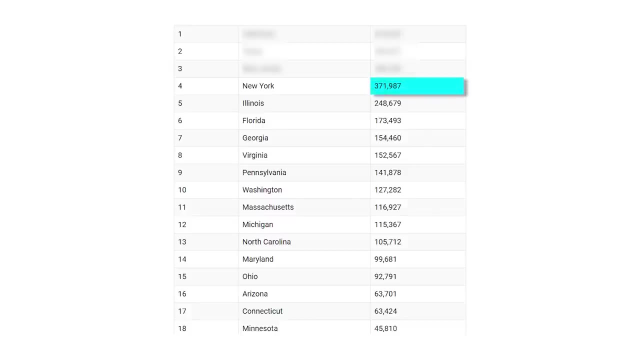 Indian student population. Indian professionals in the region find work in sciences, medicine, computer science and management. Number 4. New York. New York has the fourth largest number of Asian Indians in the US, with a total of 371,987,. 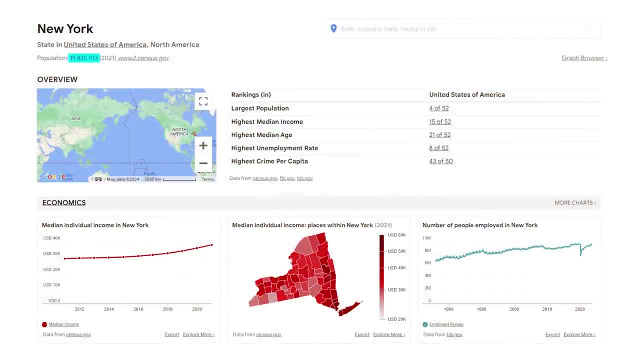 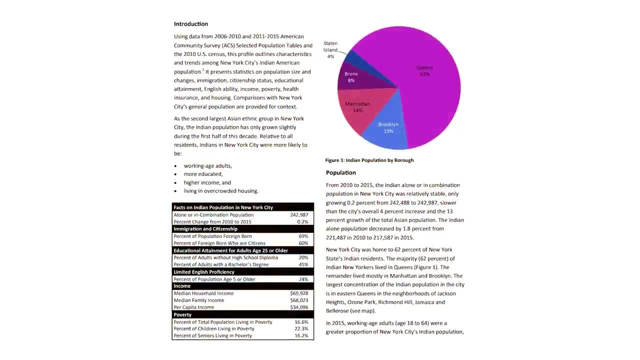 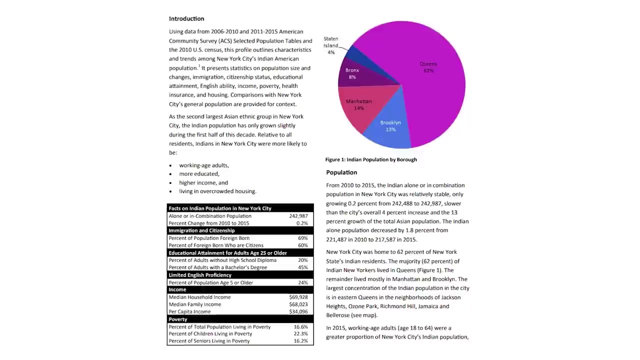 compared to New York State's population of about 19.8 million. That means that Indians make up about 1.9% of the state's population, Though when you consider that a large number of these people are in the New York City region, that percentage actually appears higher. Speaking of New York, 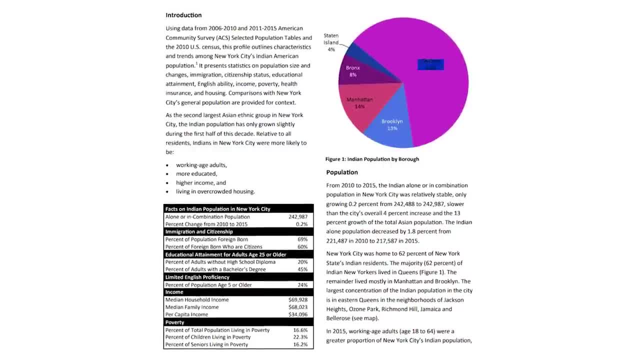 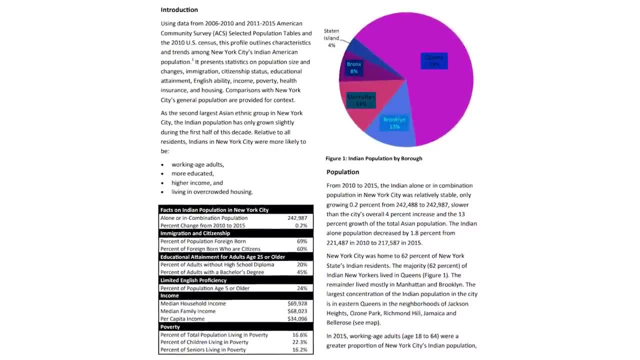 City. of the city's Indian American population, 62% live in Queens, followed by 14% in Manhattan, 13% in Brooklyn, 8% in the Bronx and 4% in Staten Island. I will note that data is from: an older census count, although it's unlikely that these statistics have changed dramatically. Compared to other New Yorkers, New York City's Indian population tends to be more educated, having a higher overall income and have a lower rate of poverty. Number 3. New Jersey. 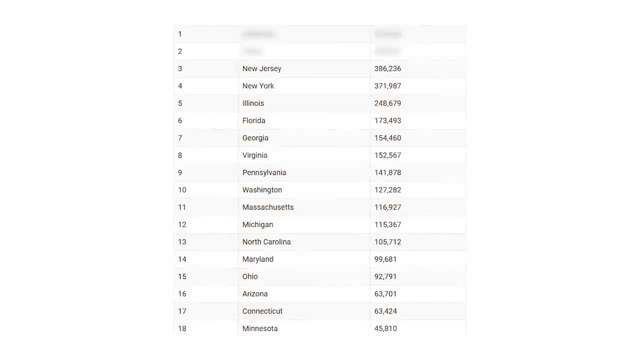 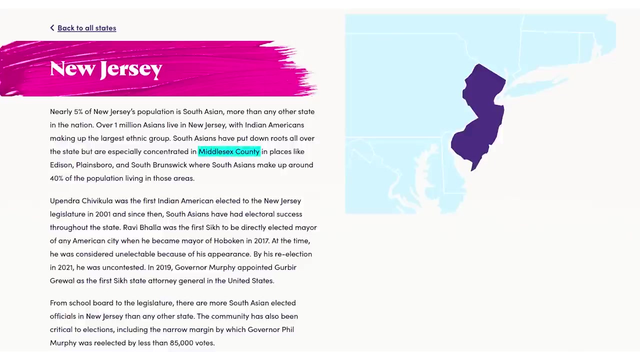 Just across the river from New York City is New Jersey, which also has a large Indian population, with 386,236 Indian residents. Most of these people live in Middlesex County, which is also, coincidentally, right across the river from New York City. 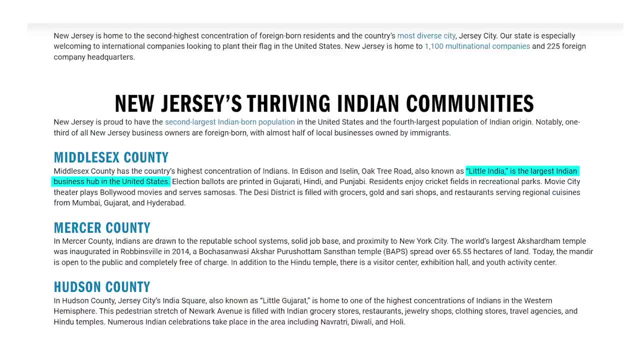 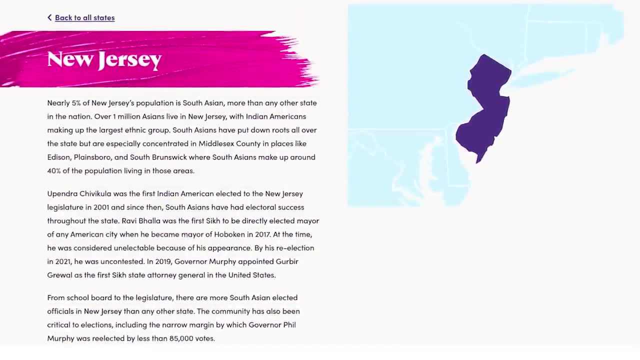 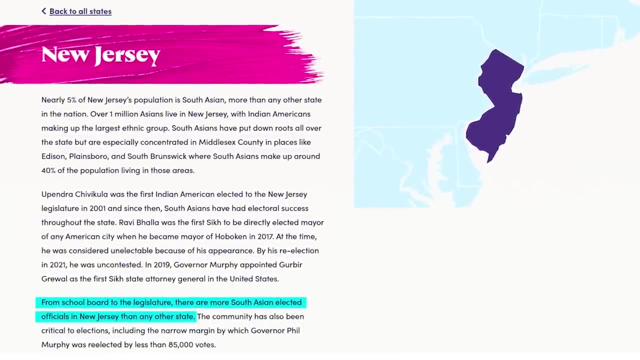 There you can find areas like Little India, which has one of the biggest hubs of Indian businesses in the US. Interestingly, South Asians, including Asian Indians living in New Jersey, are very involved in politics, with more South Asian elected officials located in New Jersey. 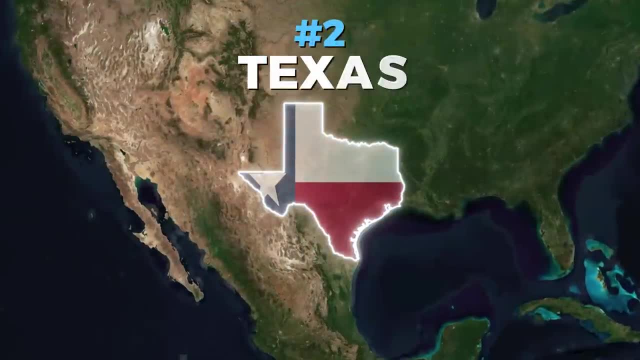 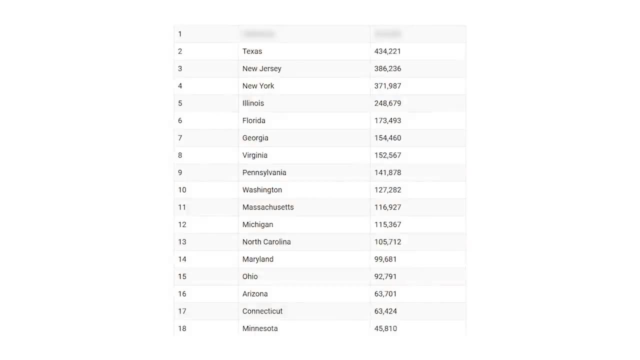 than in any other state in the country. Number 2. Texas. Number 2 on our list is Texas. Here, the Indian population is just under half a million people, with a total of 434,221.. While that might seem like a lot, it's not exactly the same as the rest of the country. 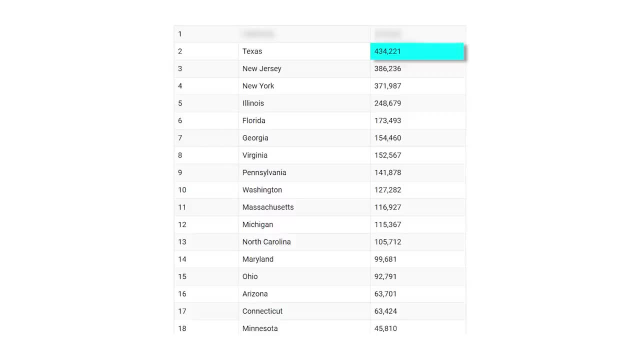 Number 2. Texas. Number 2 on our list is Texas. Here, the Indian population is just under half a million people, with a total of 434,221.. While that might seem like a lot, it's actually a little lower than some of the other states on this list. 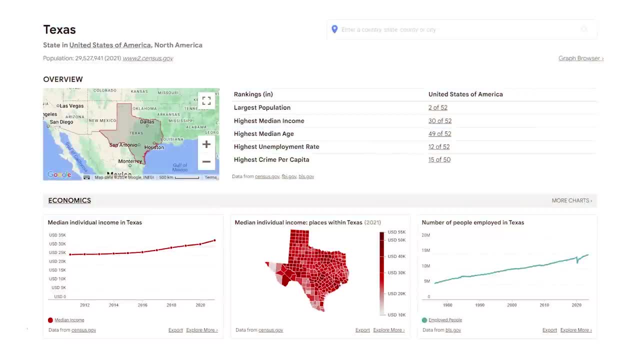 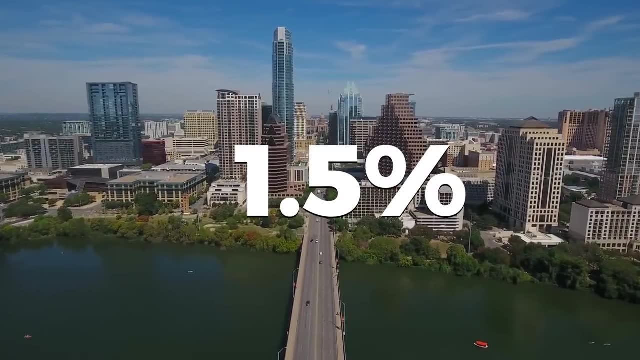 That's because Texas has the second largest population in the US, with 29.5 million people, meaning that Asian Indians only make up 1.5% of its population. Still, that doesn't mean that the number of Indians living here is small. 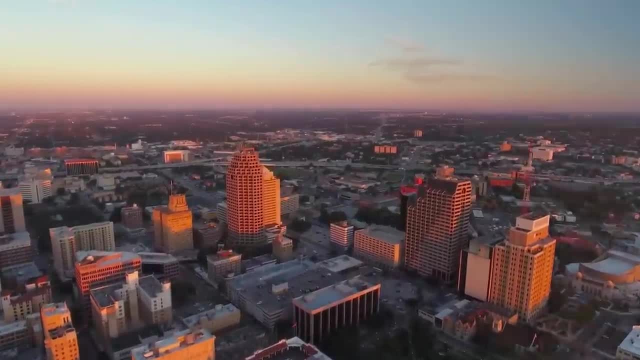 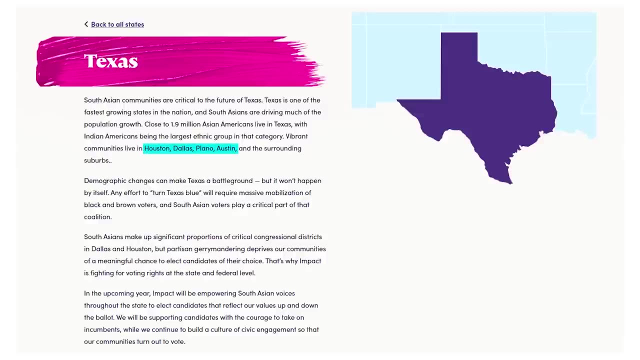 So where do most Asian Indians live in Texas? Well, like we've seen in other states, many, Many of them live in urban areas like Houston, Dallas, Plano and Austin. Like we saw with some of the other places on this list, Texas' Indian population started. 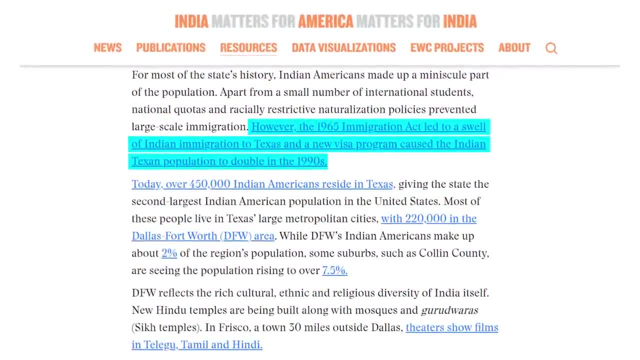 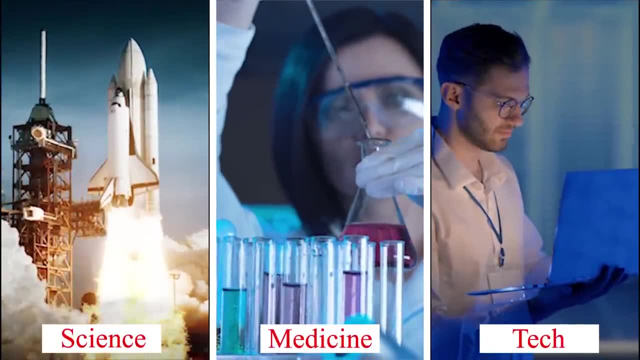 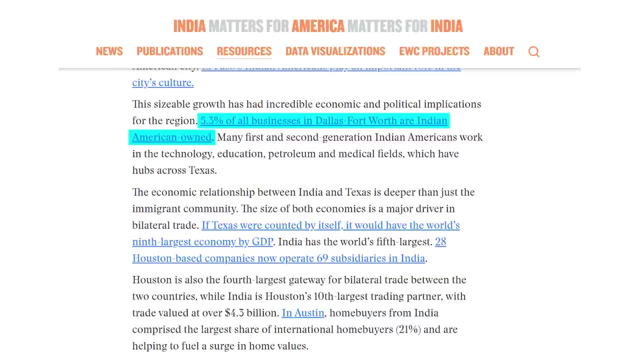 increasing after the 1965 Immigration Act and while many Indians located in Texas today are in science, medicine and tech jobs, like we've seen elsewhere, there are also a fair number of Indian-owned businesses, with 5.3% of all businesses in the Dallas-Fort Worth. 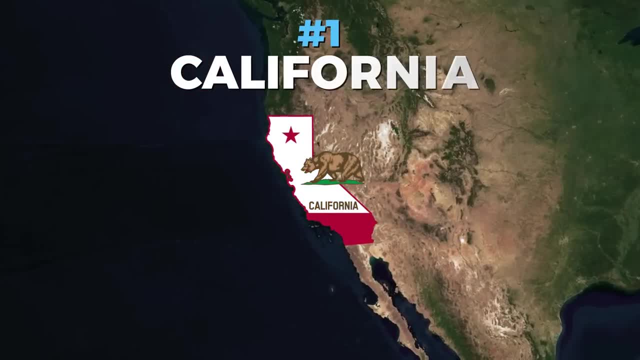 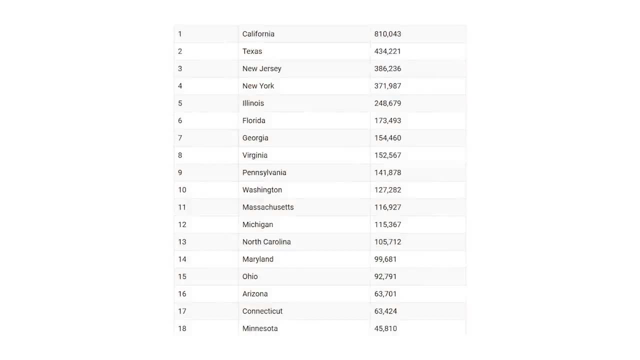 area being Indian American-owned Number 1, California. Number 1 on our list of states with the largest populations of Asian Indians is California. Here there are nearly double the number of Indians as we saw in Texas, with a total population of 810,043 people. 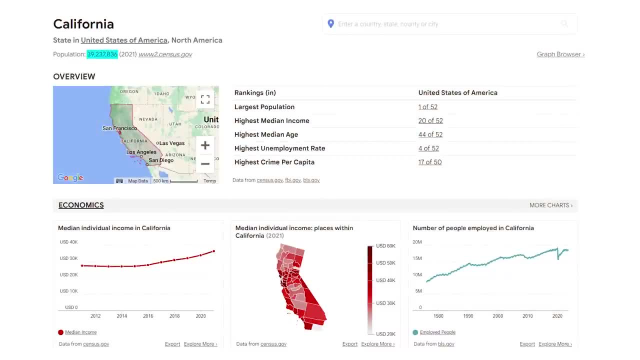 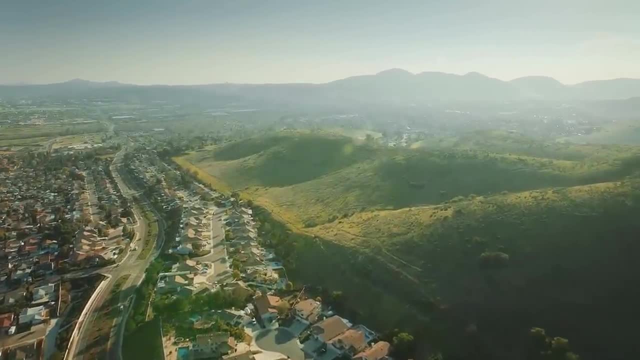 And despite California's large population, the number of Indians in the Dallas-Fort Worth area of about 39.24 million, Asian Indians actually make up a significant portion of the population here, at least relative to other states, at about 2%. 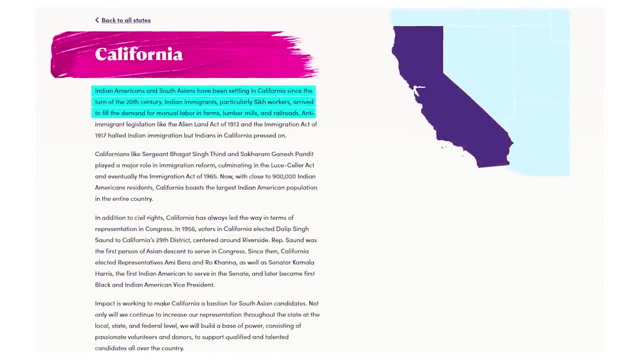 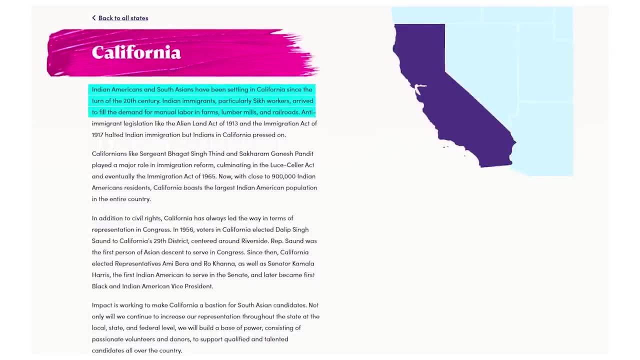 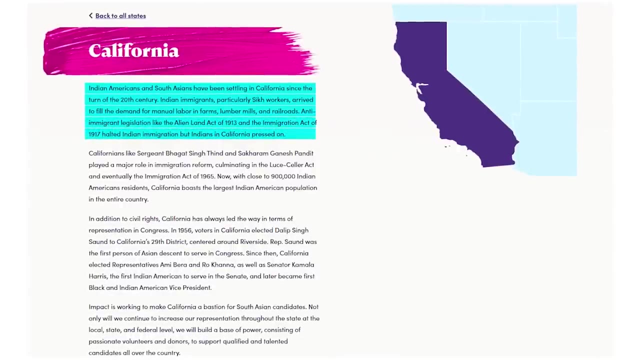 Interestingly, Asian Indians and South Asians began coming to California at the beginning of the 20th century to find work opportunities in the farm, lumber and railroad industries, After a brief decline in this number due to anti-immigrant policies enacted in the 1900s. 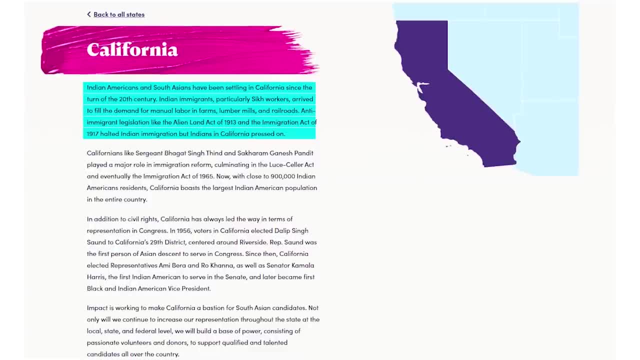 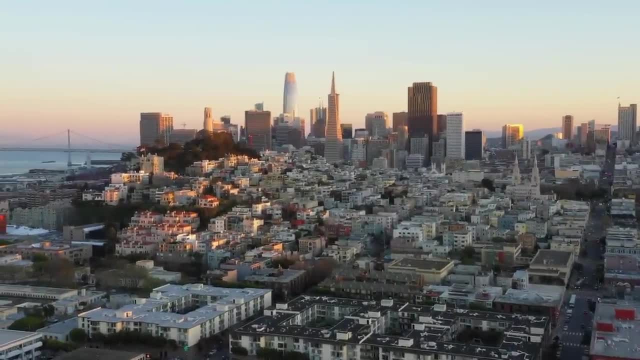 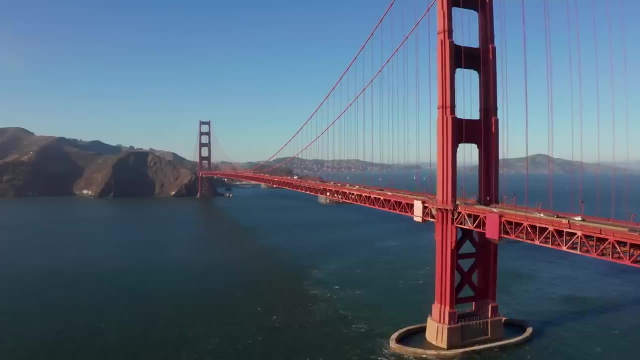 the Immigration Act of 1965 led to a resurgence in the number of Indians settling in California. Today, most of these people have settled in the San Francisco Bay area, which has also seen the highest growth in its East Asian population. What about the states with the most illegal immigrants? 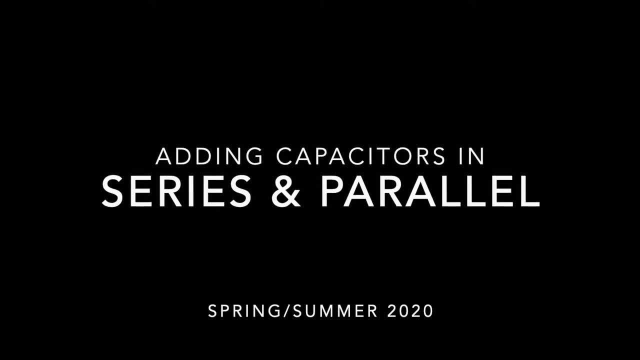 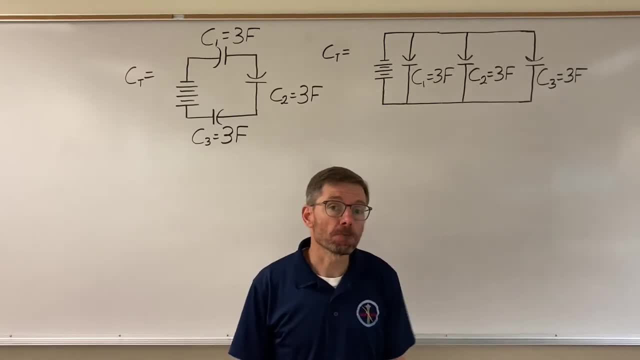 Today we'll be adding capacitors in series and in parallel. So how do we add them? First of all, a capacitor. its capacitance is measured in farads, And I've got three capacitors here: three farads, three farads, three farads and the same here, three, three and three. These are in. 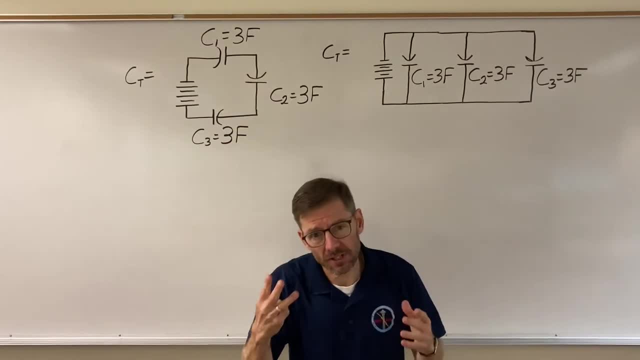 series and parallel. Now I understand. three farads is a huge amount. When we're working with capacitors, they're generally going to be in the microfarad or nanofarad range. So why did I use whole numbers? Just so we're not dealing with the exponential math. We're just 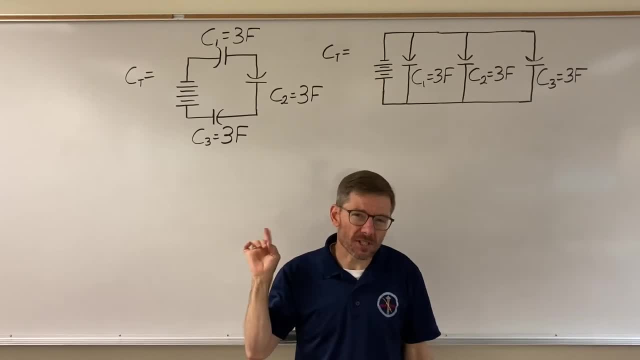 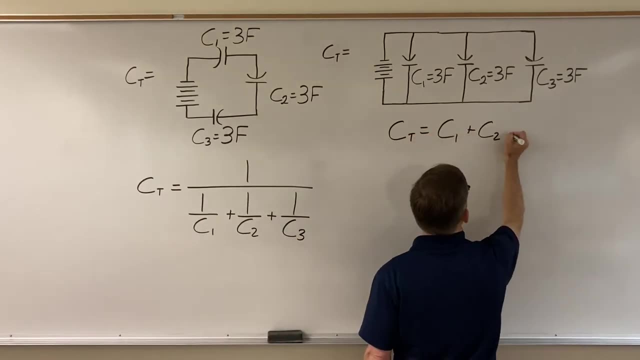 looking at the concepts as to why these formulas that I'm going to write up are actually the case. Did I mess up with these? We're used to seeing this formula for adding resistors or inductors in parallel and this formula in series, But part of this has to do with the nature of the capacitor. 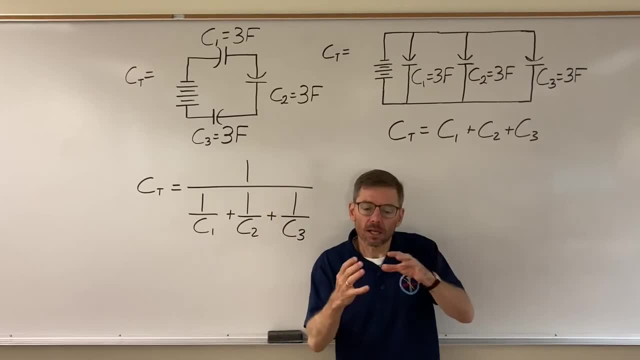 This is actually correct, as is this: Capacitors can be seen as complementary to inductors. Okay, so we're going to find that a lot of the math is upside down. The vectors where an inductive vector pointed up, a capacitive vector points.